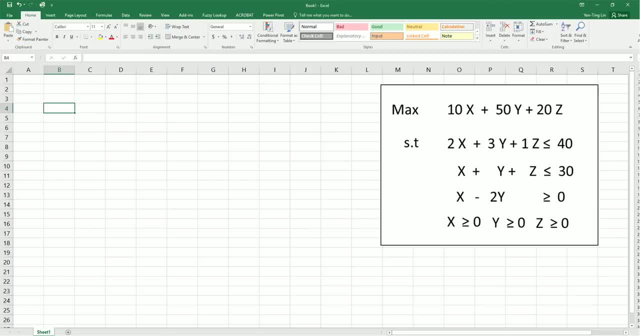 Here I'm going to show you how to use Excel Solver. Let's suppose that we have this problem to optimize. Here's the objective function over here, with three decision variables: x, y and z. We want to maximize this function subject to those. 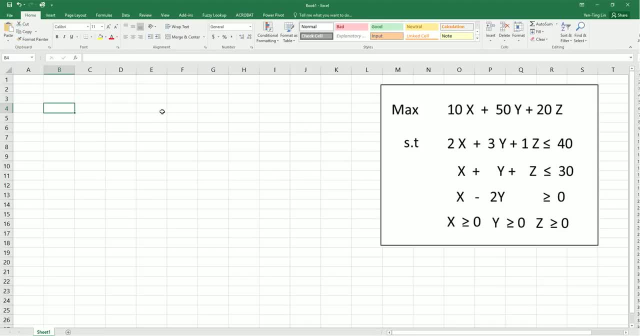 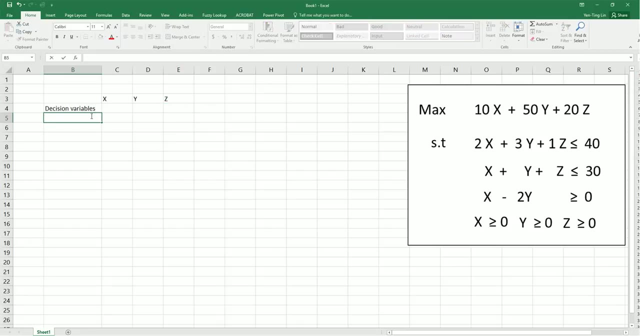 constraints. Now let's start by defining decision variables. Okay, we have x, y and z. Now let's go here. Okay, and now let's store the value of those decision variables here. and coefficients: Coefficient for x is 10, for y is 50, for z is 20 in the objective function. So we put: 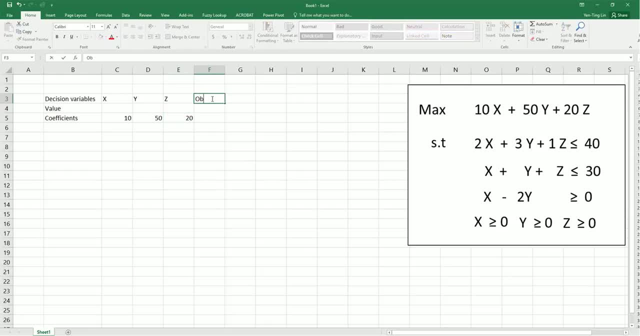 them here. Objective value: okay, which is the value of this objective function with the value of those decision variables? over here, Let's put one, one one as a placeholder in the beginning. You can put any number you like, doesn't matter. 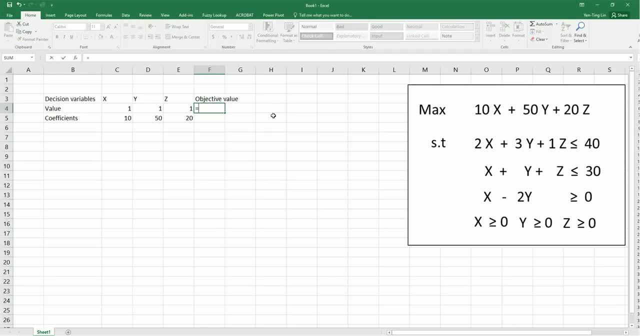 Okay, Okay. Okay, So we're going to use a function called SUMPRODUCT- S-U-M-P-R-O-D-U-C-T- SUMPRODUCT. First input is the array for decision values. Second array is the coefficients. Okay, so it will do 1 times 10 plus 1 times 50 plus 1 times 20.. Okay, So we're. 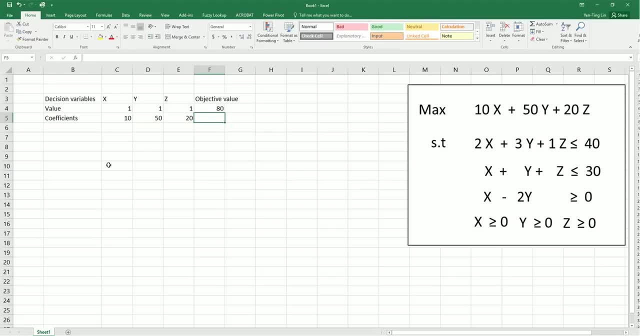 done Now with the objective function. now let's key in constraints. Let's give the constraints names: Constraint 1,, 2, and 3. It's very helpful to give them names because later on in the sensitivity report the report will use those names, so you know which constraint 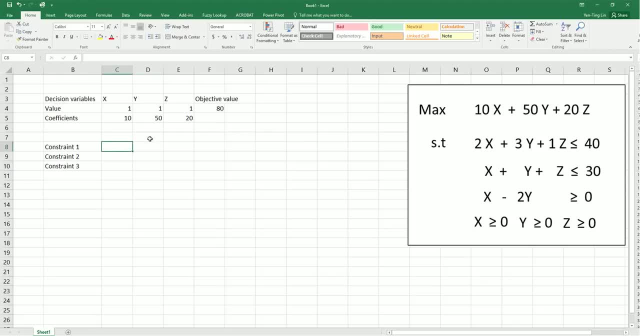 you're talking about, For each constraint, let's say constraint 2, constraint 3,, constraint 1.. We just key in the coefficients for the decision variables, So 2,, 3, and 1. And here we store something called LHS and RHS. LHS stands for left-hand side, RHS stands for 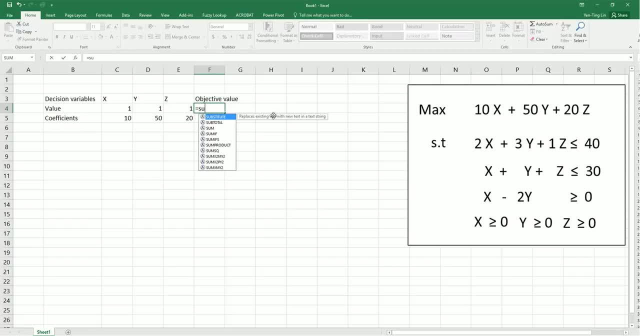 So we're going to use a function called SUMPRODUCT- S-U-M-P-R-O-D-U-C-T- SUMPRODUCT. the first input is the array for decision values. Second array is the coefficients. So it will do 1 times 10 plus 1 times 50 plus 1 times 20.. 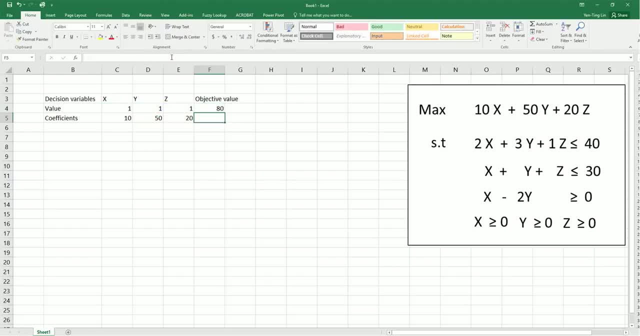 So we're done with the objective function. now let's key in constraints. Let's give the constraints names: Constraints 1,, 2, and 3.. It's very helpful to give them names because later on in the sensitivity report, the report will use those names. So you know you're going to use the names that are in the sensitivity report. So you know you're going to use the names that are in the sensitivity report. So you know you need to keep those names in mind so you can see exactly which constraint you're talking about. 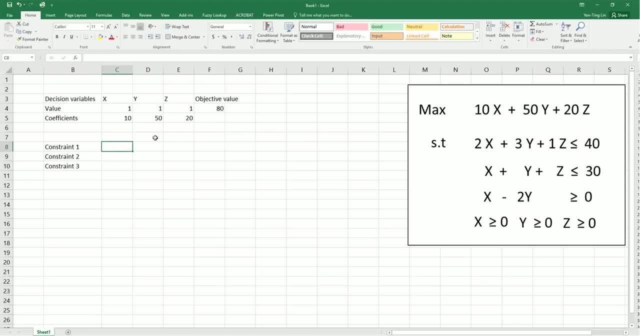 For each constraint, let's say constraint 1,. for each constraint, let's say constraint 1, we just key in the coefficients for the decision variables, So 2,, 3, and 1.. Here we store something called LHS and RHS. 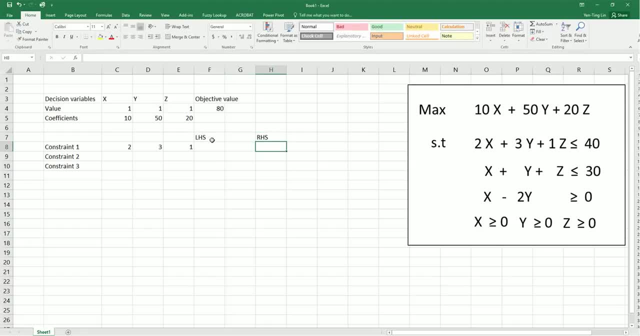 Here we store something called LHS and RHS. LHS stands for left hand side, RHS stands for right hand side. So it's a left hand side and right hand side value of the inequalities I give a less equal to, because The first constraint is less equal to what? 40. So I keep 40 over here for right hand side value. Left hand side value is the calculation of this 2x plus 3y plus 1z, using the decision values over here. 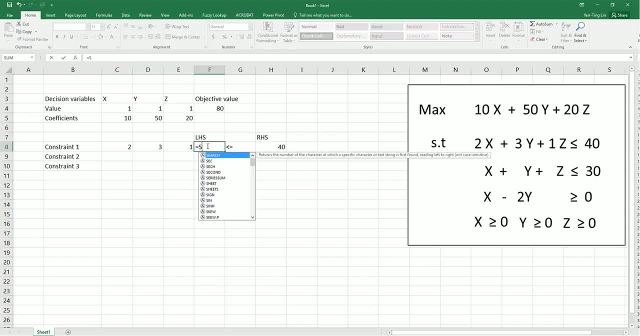 So how do we calculate that? Again, some product. Okay, this array multiplies this array. But now I'm going to put dollar sign for this array because then I can drag it down. If you're using a PC, you just move your cursor and click on it anywhere in this C4 and then press F4. 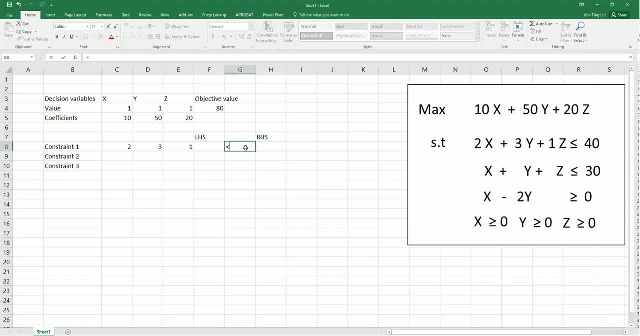 right-hand side. So it's a left-hand side and right-hand side value of the inequalities. I give a less equal to, because the first constraint is less. equal to Less, equal to less. equal to what: 40.. Okay, so I'll key in 40 over here for right-hand side value, Left-hand. 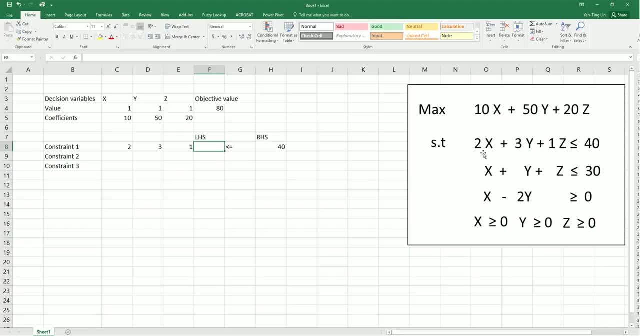 side value is the calculation of this: Two x plus three y plus 1z, using the decision values over here. So how do you calculate that? Again, sum product. Okay, this array multiplies this array. Okay, so that's the product. Okay, Now let's do the same thing. 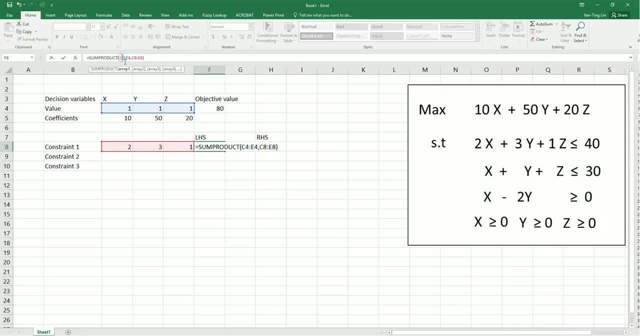 let's do the same thing Again: sum product: This array multiplies this array. Let's give. But now I'm going to put dollar sign for this array, because then I can drag it down. If you are using a PC, you just move your cursor and click on it anywhere in this C4 and then press F4. 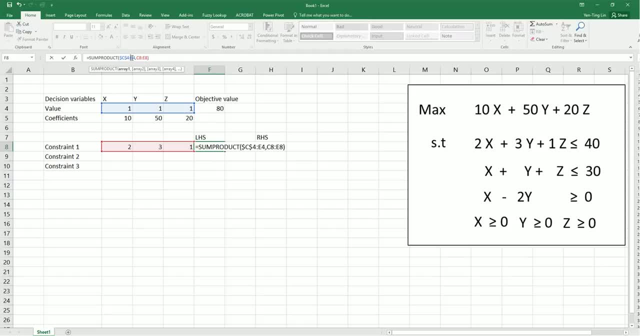 Okay, now you have dollar sign. Now you move your cursor to E4 and press F4.. Okay, so now you fix a reference to C4 to E4.. Now we have the first constraint done. So what it means here is that the left hand side value for this constraint is currently 40.. 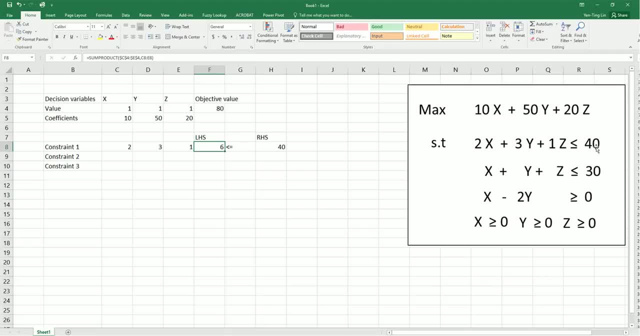 In the optimum, it needs to be less than 40.. Sorry, let me correct that. For the current decision variables, the left hand side value is 6.. In the end, it needs to be less than 40.. Okay, now we can move on to constraint 2.. 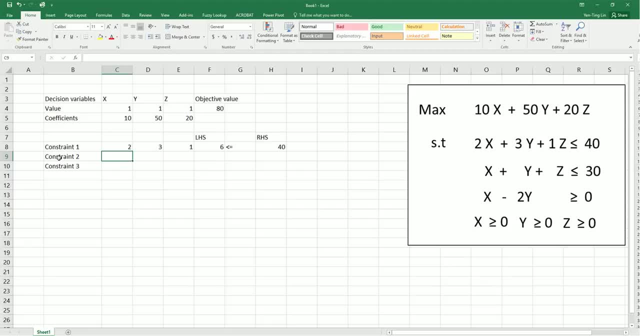 The coefficients are 1,, 1, and 1.. Okay, 1,, 1, and 1.. Still less, or equal to right hand side is 30. For left hand side value, we can just drag it down now. 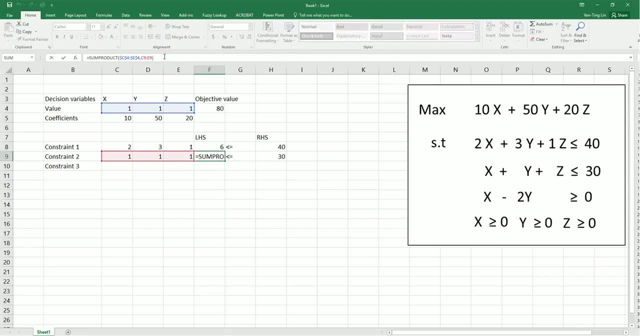 And you can see it's the correct calculation. Last constraint: the coefficients are 1, minus 2, and 0. You can leave it blank if it is a 0.. Left hand side value: Just copy the formula, But now the sign is larger or equal to greater or equal to right hand side value is 0.. 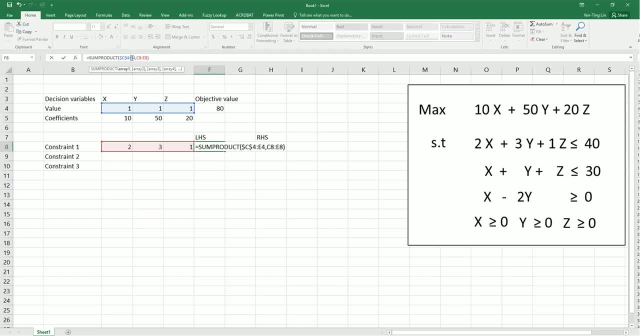 Okay, now you have dollar sign. Now you move your cursor to E4 and press F4.. Okay, so now you fix a reference to C4 to E4.. Now we have the first constraint done. So what it means here is that the left hand side value for this constraint is currently 40. In the optimum it needs to be less than 40.. Sorry, let me correct that. 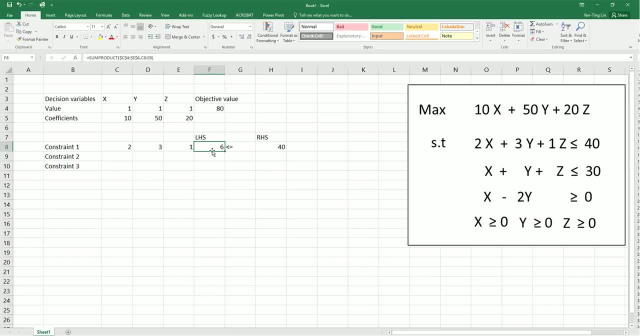 For the current decision variables. the left hand side value is 40.. The left hand side value is 6.. In the end, it needs to be less than 40.. Okay, now we can move on to constraint 2.. The coefficients are 1,, 1, and 1.. Okay, 1,, 1, and 1.. Still less, or equal to right hand side is 30.. 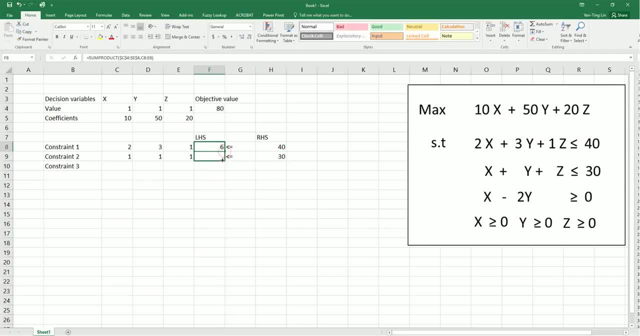 For left hand side value. we can just drag it down now And you can see it's the correct calculation constraint. the coefficients are 1, minus 2, and 0. You can leave it blank if it is a 0.. 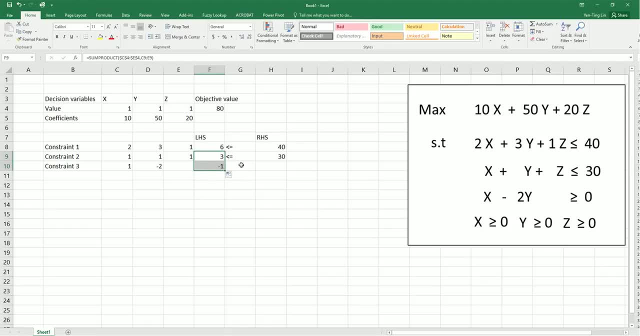 Left-hand side value. just copy the formula. But now the sign is larger or equal to greater or equal to right-hand side value is 0.. So basically, that is the input of the formulation. Now let's open up Solver right here. 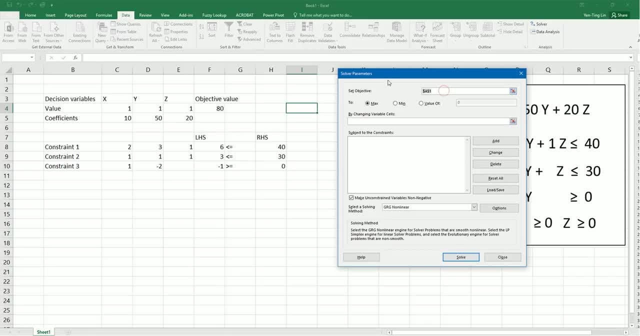 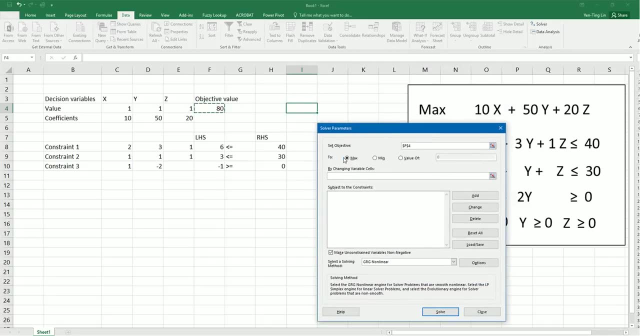 The objective so set objective is the value we try to maximize or minimize. In this case it's here. We want to maximize this value, so you click Max. If you try to minimize it, you click on Min Here by changing value cells. so these are the cells that you allow Excel to change. 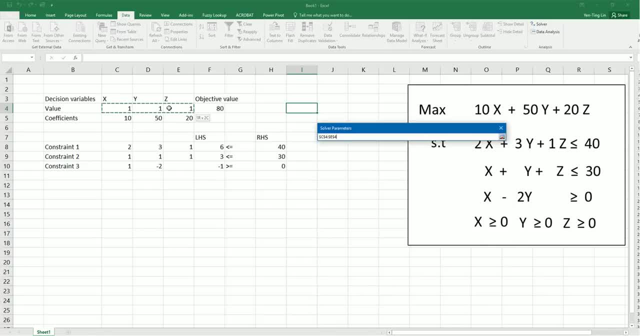 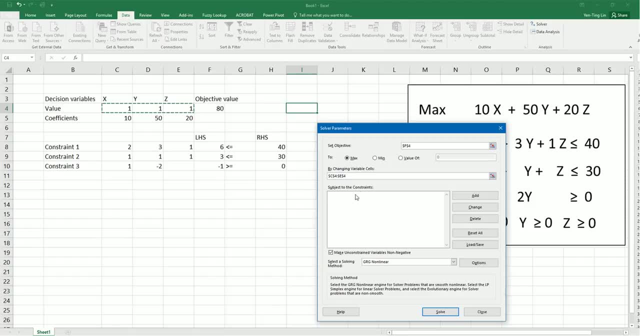 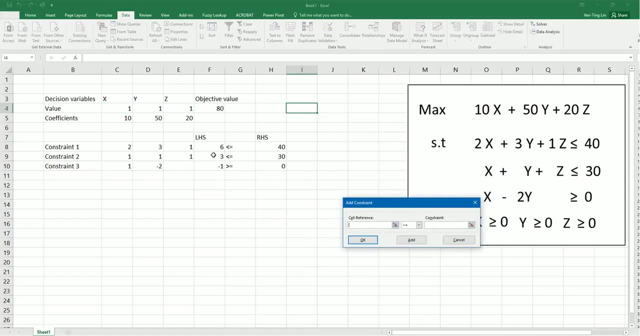 So, which means that these are the decision variables. So just select these three cells, because these are our decision variables. you need Excel to find the optimal value for Constraints, so let's add. click on Add to add a constraint. These two constraints have the same sign. 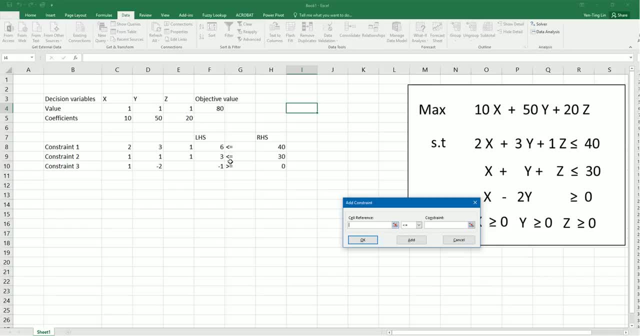 Both are less or equal to. So here you can just select these two. It will go here. Okay, It means that the left-hand side value should be whatever, In this case less or equal to. here You give it the right-hand side value. 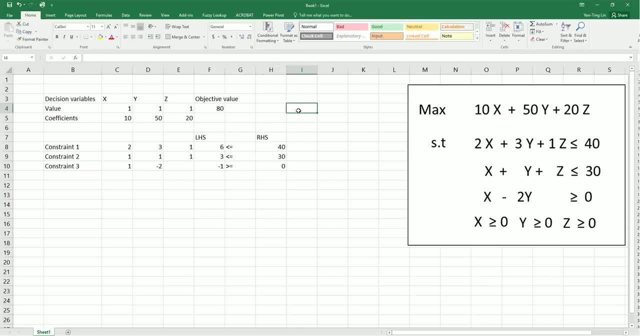 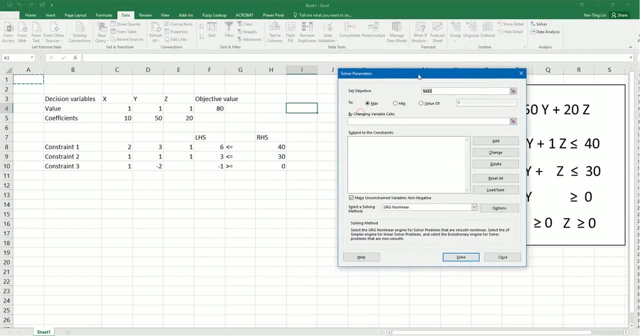 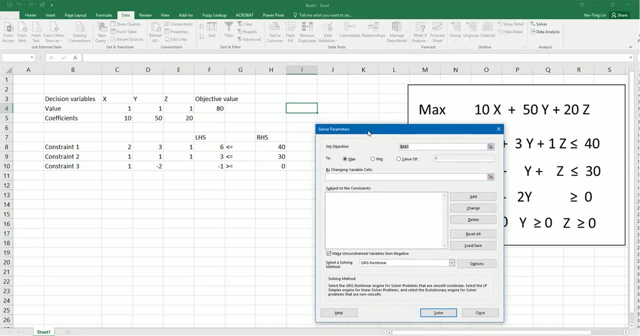 So basically, that is the input of the formulation. Now let's open up solver Right here. The objective, So set objective, is the value we try to maximize or minimize. In this case, it's here We want to minimize, We want to maximize this value. 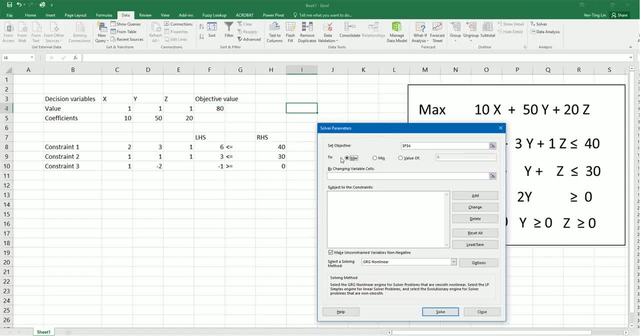 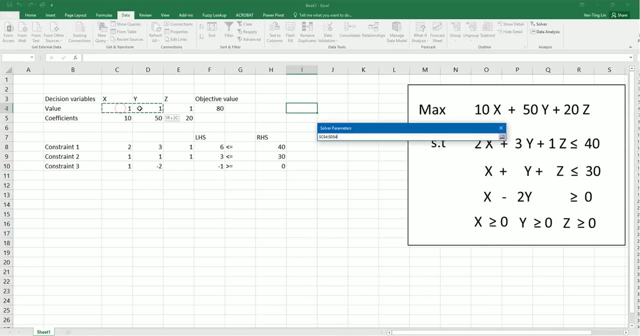 So you click max. If you try to minimize it, you click on mean Here by changing value cells. So these are the cells that you allow Excel to change. So which means that these are the decision variables. So just select these three cells, because these are our decision variables. 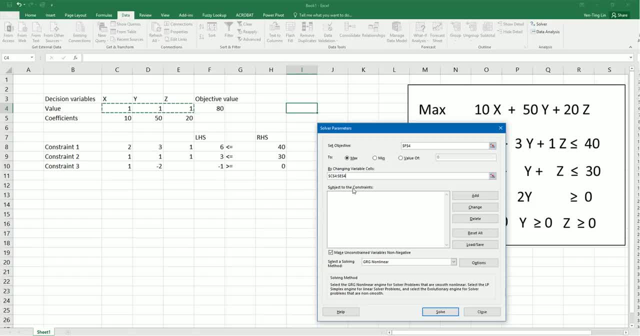 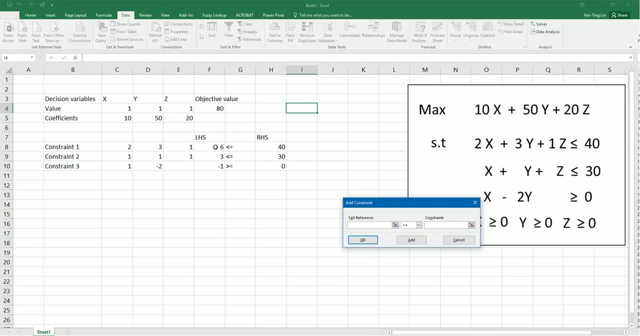 You need Excel to find the optimal value for Constraints. So let's add. Click on add to add a constraint. These two constraints have the same sign. Both are less or equal to. So here you can just select these two. It will go here: 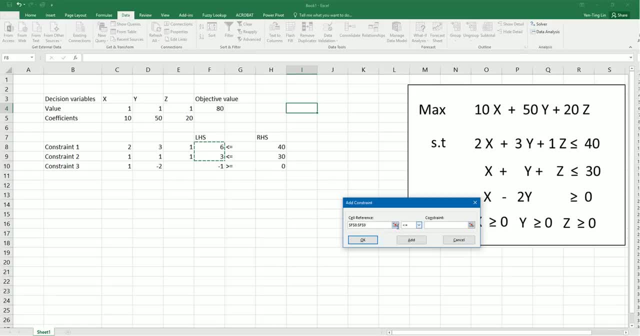 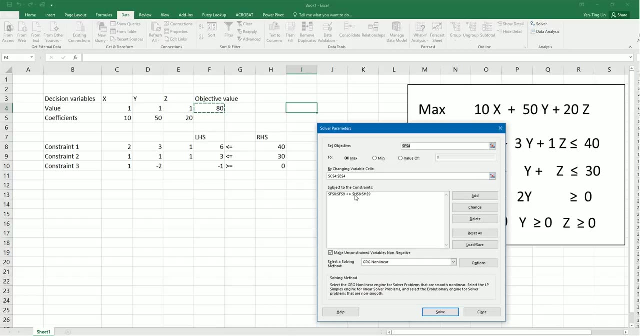 It means that the left hand side value should be whatever, In this case less or equal to here. You give it the right hand side value. OK, So we add one set of constraints. Actually, this combines two constraints: Constraint one and two. 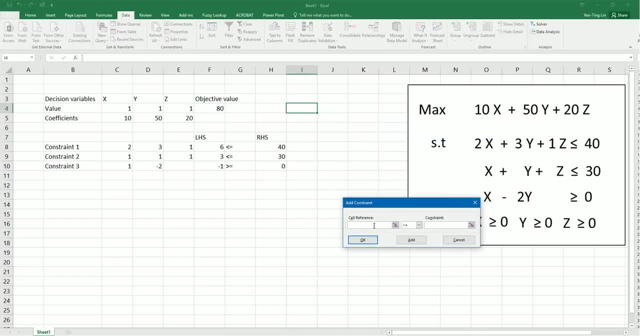 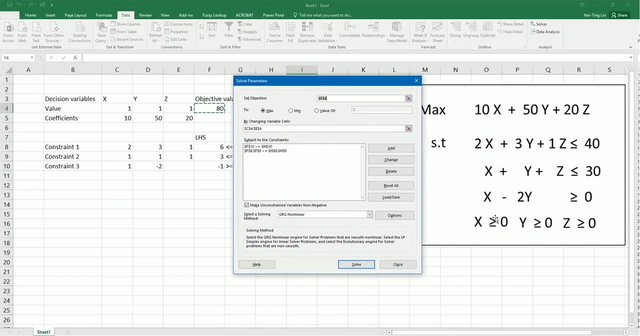 Now let's add another one for constraint three. Left hand side value need to be, in this case, greater or equal to the right hand side value. OK, And we actually have three non-negative constraints. So if we add a constraint, say that x and y and z cannot be negative values. 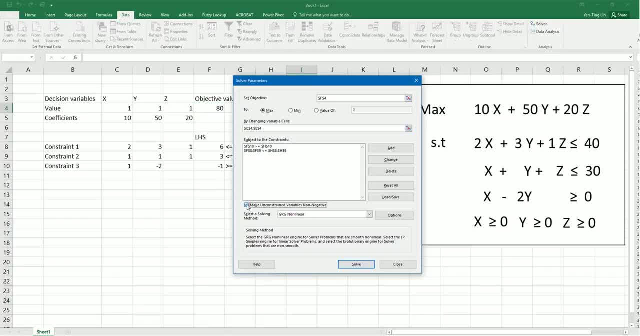 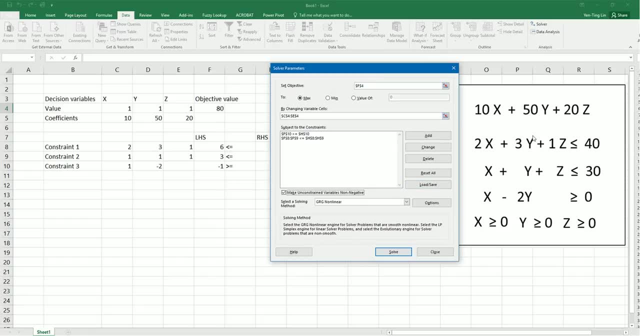 You can include that constraint by just clicking checking this checkbox. And if your problem is a linear programming problem, which means that every expression is linear in the decision variables, Then you can just go for simplex LP. But if your problem is not linear,